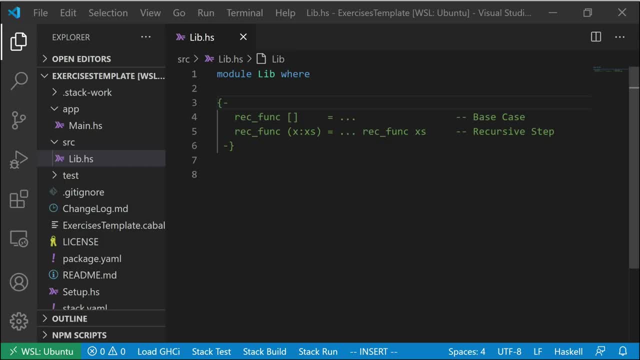 rest of the list here. All right, let's actually take a look at some examples of functions that use this pattern of iterate through a list, you know, one element at a time, recurse and do something at the empty list, return some value. So 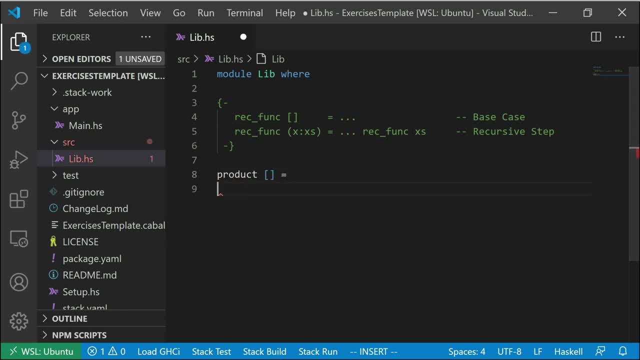 Prada is a function that's going to take a list and multiply every element inside that list together. So the way it's going to work is we're going to iterate one thing, one time list. So we're going to have this pattern. I'll put it here to fill in. Okay, we need to fill in these dot dots. 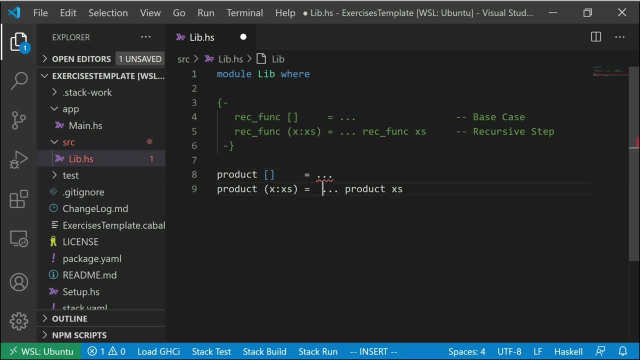 here. So what we're going to do is we're going to pull out each of these elements and then we're going to take this element of the list and we're going to multiply it against the product of the rest of the list And at the base case. so if we, if we follow, if we started the recursive step and 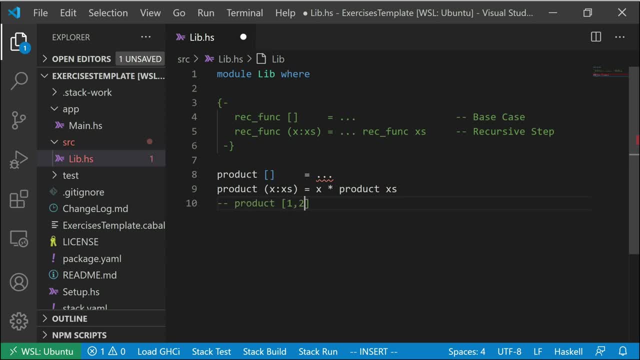 we run through the evaluation of it, we're gonna have product of, let's say, the list one two. And remember the list one two is the same, that that's just a special way of writing one colon, two colon, empty list. 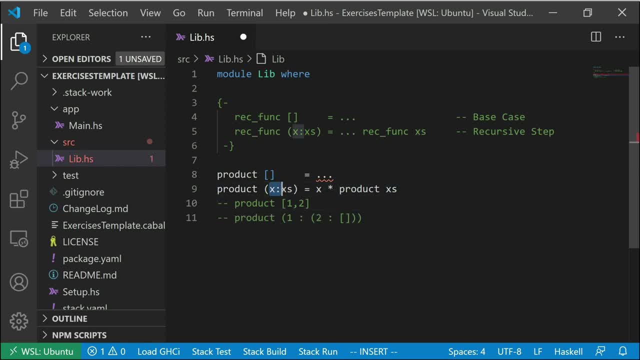 This is going to pattern match to this case here. okay, where x is one And x is is two, colon empty list here And this will evaluate. so running one step of evaluation here, it's going to become one times product to colon empty list And of course now we do the same thing for the next product. 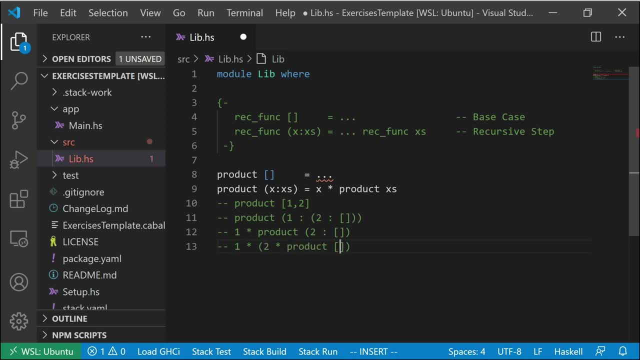 and we end up with two times product to us. Now you'll see what we already wanted to accomplish is like already done here. Okay, so we're already kind of finished our work by the time we get to the empty list. So what we need now is something to multiply against. that isn't going to change what we've. 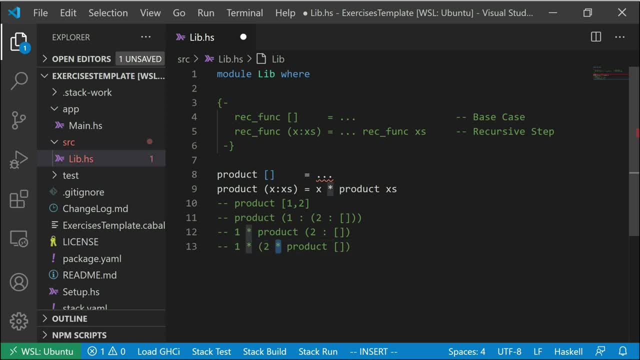 already done And, of course, everybody should be able to figure out. if you multiply something by one, Okay, that should leave everything the same. So then this becomes one times two, times one, of course, times two. Okay, you may have noticed right now, if you, if you try and load into GHCI. 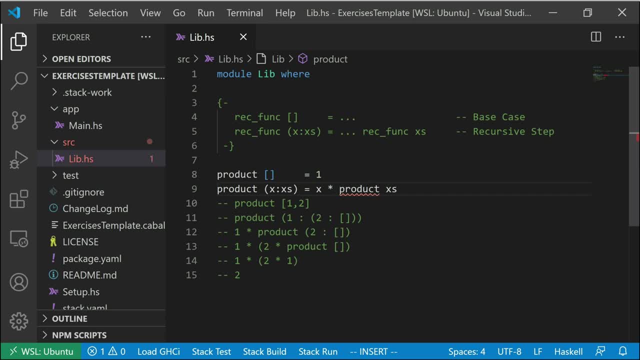 that product. here it's giving us an error because product already exists inside the prelude, So we can't define product twice. we could just change the name of it, which I'm sure you guys have been doing when running through some of the exercises I've given. But here's a handy little trick. 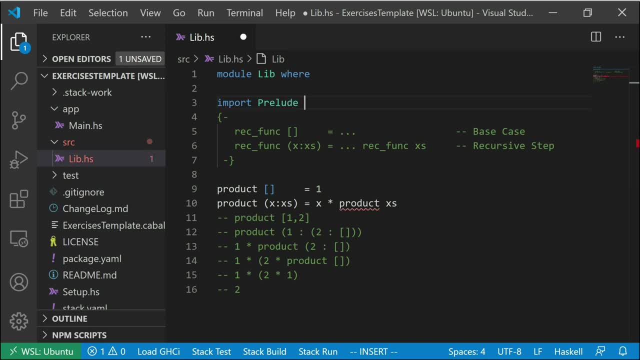 We could import the prelude explicitly. So usually this is kind of like just already done here by default. But then we could use this- a nice little thing that has to do. we say hiding, and we could hide the product from the prelude And this way it no longer gives us an error because we're no longer importing the. 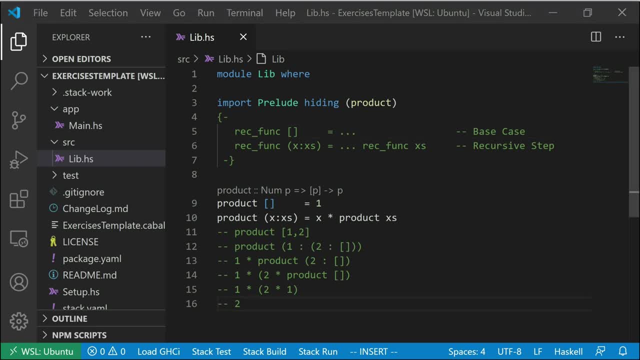 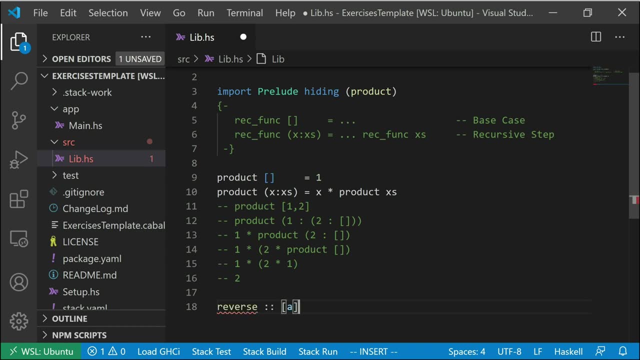 product. that comes from the prelude. Pretty cool. Let's do another example. So reverse is going to be a function that's going to take a list and return another list. is going to be that same list, but every element is reversed. So reverse- empty list is going to equal something, And reverse x, colon x's. 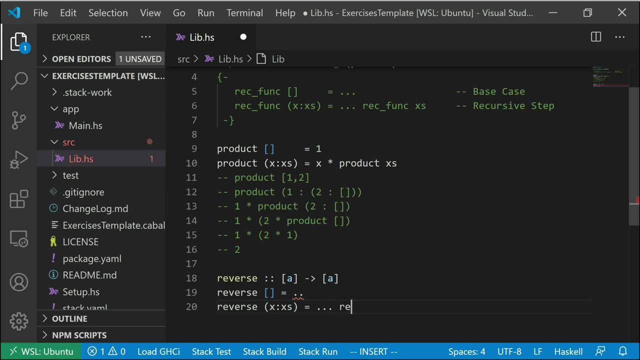 is going to equal something, And then we're going to recurse. Now one trick to reverse here: it's not going to follow this formula. A lot of that I laid out completely strictly. what we're going to do is we're going to 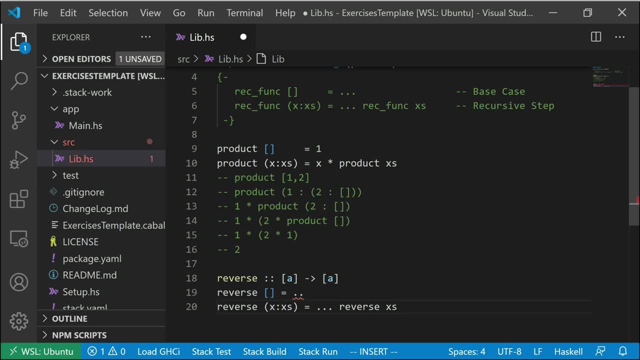 we're going to build a list with plus plus, okay, so what we're going to do is we need to take x and build another list. take the head of the list and build another list. So we're going to have x here And then we're going to put it together with the rest of the list using plus plus. 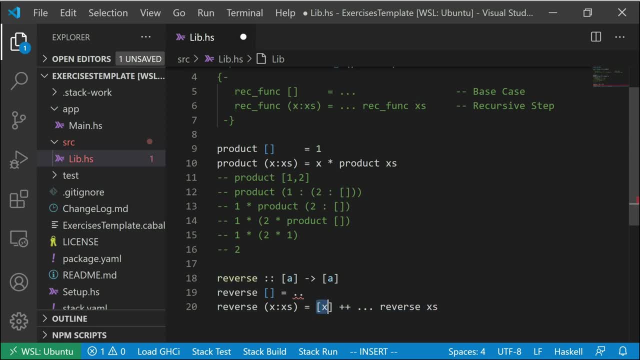 here. So we're going to put x into a list by just surrounding it with brackets. So now it's the single list of x. we're going to add it. Okay, put it together with the reverse of the other list. But here's the trick. here, If x is, 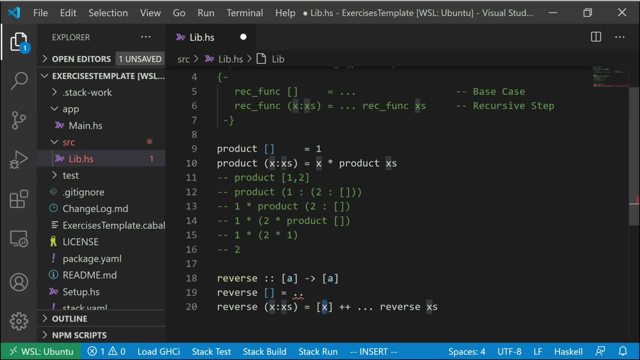 the first thing on the list, then it needs to be put at the back of the new list, right? So we need to do this in the reverse order. So said we'll do the reverses of x's plus plus x here, And we're going to keep doing this. 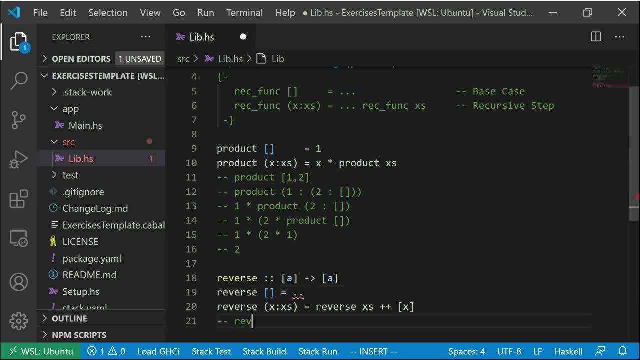 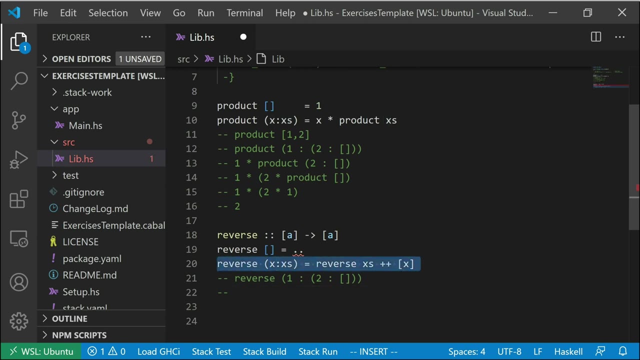 Okay, so you run through the little evaluation here We have reverse of, say, one empty list again. So this is going to pattern match to this case where one is x here And we're going to end up with reverse to empty lists plus plus one, which is going to become what? well, that's going to. 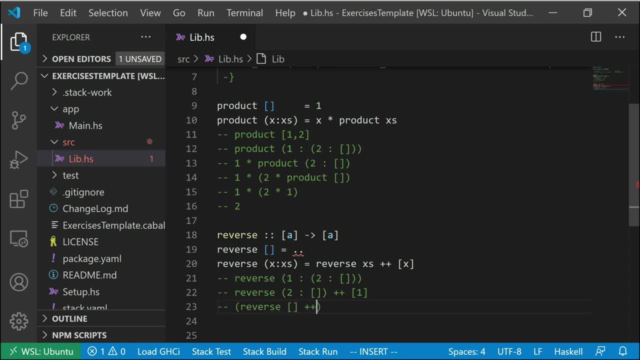 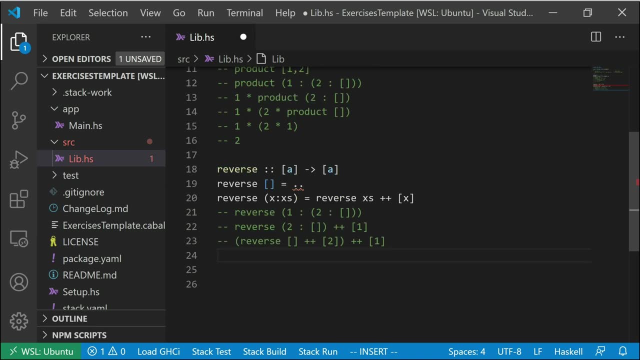 become the reverse of empty lists plus plus one, Plus plus list of two plus plus one, And then what do we want to return? an empty list. So once again, it's the same thing as before when we add the list of one and two together. 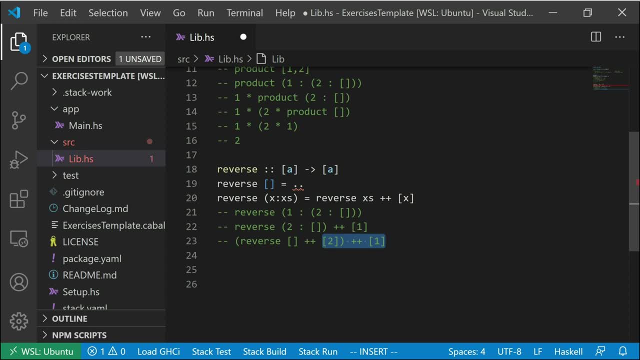 when we put these lists together to make one list. we're already done And, once again, we just need to finish this off with something that's not going to change the work. we've already done. So for the empty list and plus plus. here we're going to use the empty list. 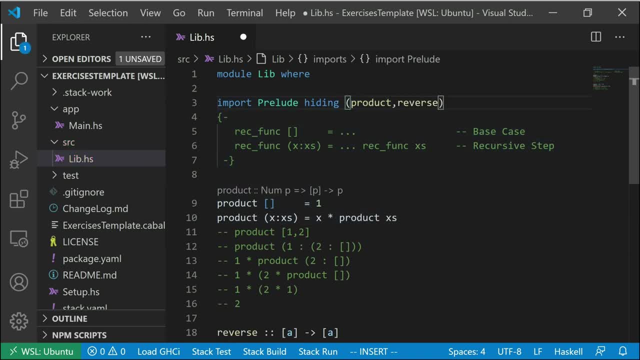 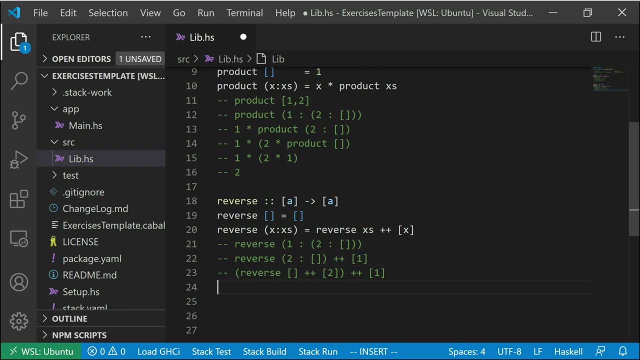 Again, reverse already exists, So we'll hide it. Okay, so this way, using the empty list, this will become the empty list plus plus two plus plus one, which will all go together to be the list of two, one which is the reverse of list two. 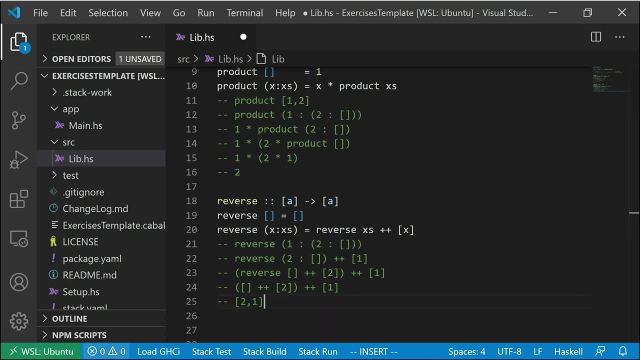 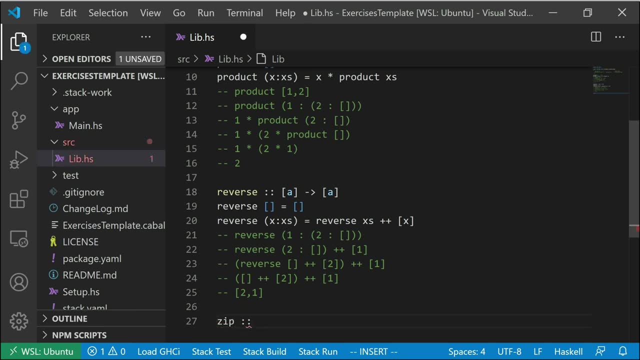 Okay, Okay, Okay, Okay, Okay, Okay, of one, two. All right, let's try a bit of a more interesting example. So zip isn't going to take just one list, It's going to take two lists, And what it's going to do is it's going to create a. 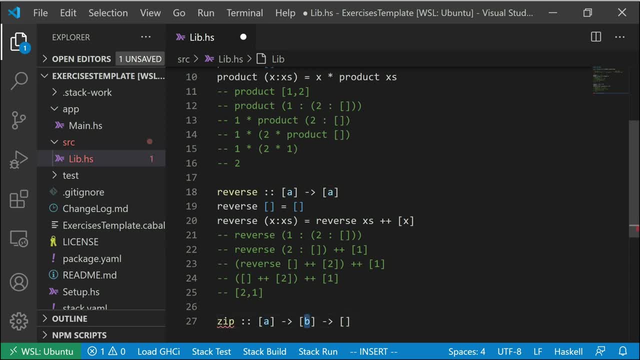 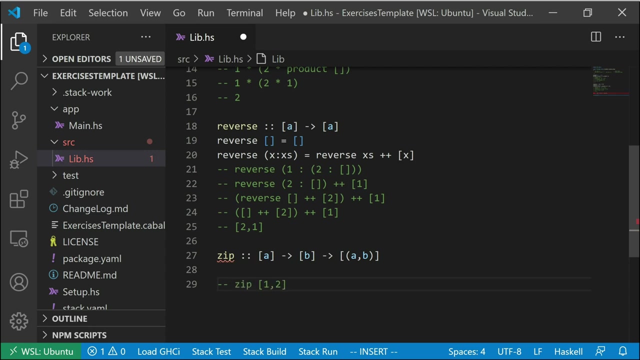 new list with each corresponding element. okay, in the two input lists put together kind of paired up in a tuple. So it's going to move to the list and it's going to pair up corresponding elements of the list into a tuple. So as an example here: zip of one to a. B should return the tuple of one a. 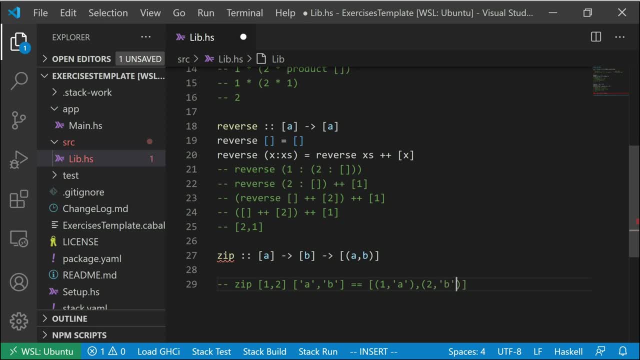 to B. Okay, now you do have to cover this scenario. Okay, what if one list is bigger than the other list? So what if you have almost the same thing, But this list is bigger? it should. it should still return the same thing. it should just stop at wherever. 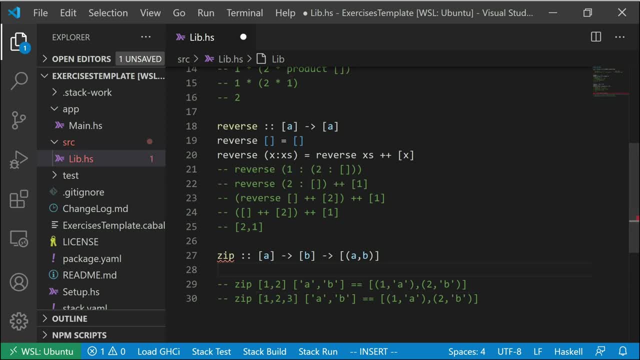 the shorter list is it'll stop pairing things together. Okay, so how would we rate set? So let's start with the recursive case. here we would have both. we have x colon x's and y colon wise. So this is assuming that there's at least one thing in each list. 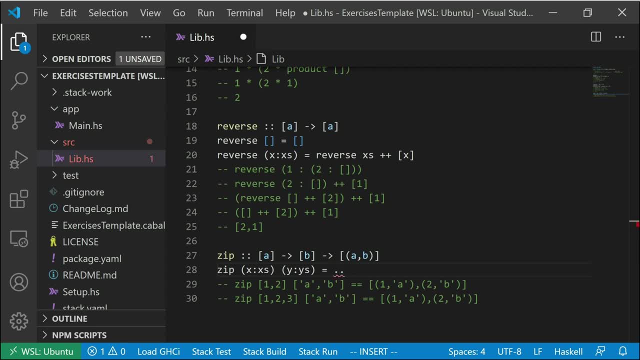 So if we do have one thing in each list, so we're gonna have to do something and then recurs on thealt of the rest of both lists, right? So if there is one thing we're going to list in any in each list, we'll pair together in a tuple, okay, and then we'll put it back into a 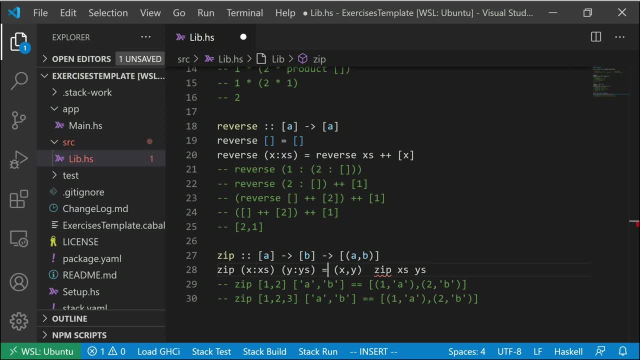 list. either we do colon or we can put it into a list and use plus plus. it doesn't matter, it's the same thing. whoops, now we need to cover the case. okay, what if these lists are empty? so you might be tempted to at first, right pattern match to both empty lists, but then you remember okay. 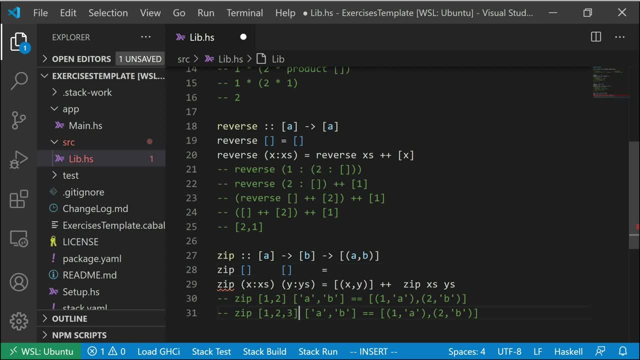 what if one is empty and the other one isn't? this case here, right? so really, what we need to pattern match to is: okay, let's time rash if this one is empty list, and then we don't care what this one is, or if this one is empty, or if we don't care what this one is, the first one is. 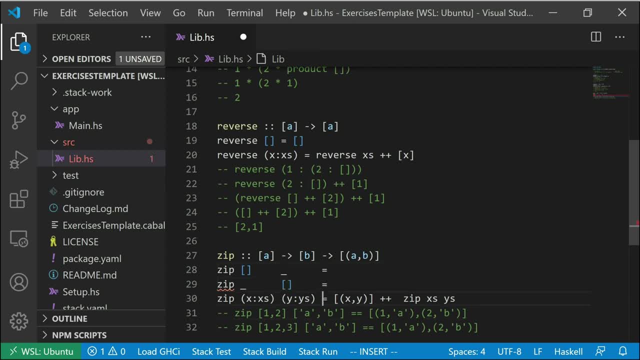 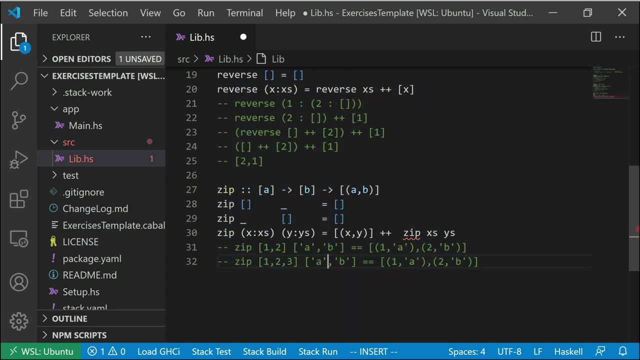 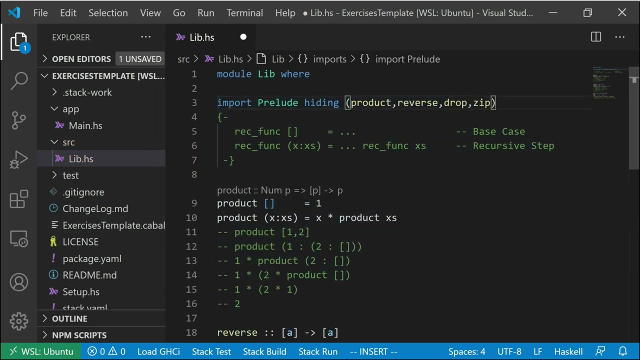 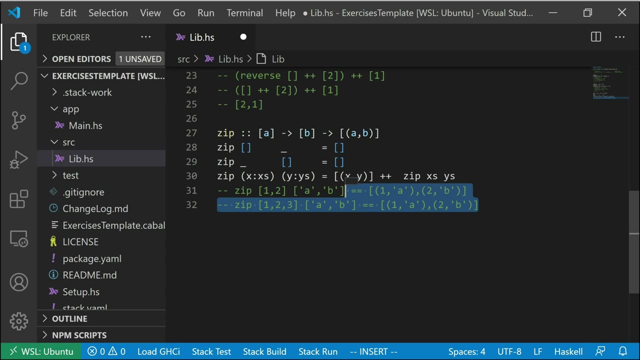 is, and this one is the empty list, and in both of these cases we can return the empty list. okay, so both of these cases will finish off and once again we'll add zip this. so if we were to run through an example of this, how would this example work here? right, zip, one colon, empty list. 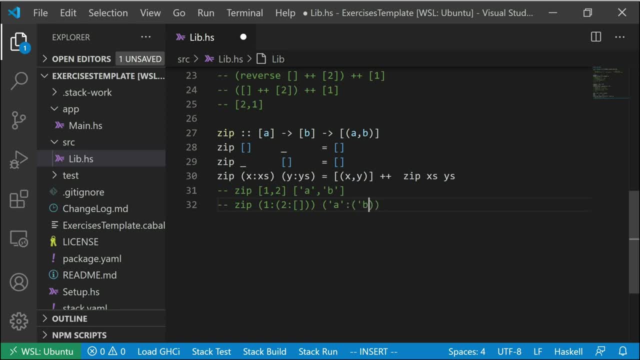 a colon b colon: empty list. okay, if we were to run through this, take one a, let's go with the example we have right now. put into a list, we plus, plus it with zip- empty list. okay, now this is going to expand, of course, to lists and then both will be the empty list. 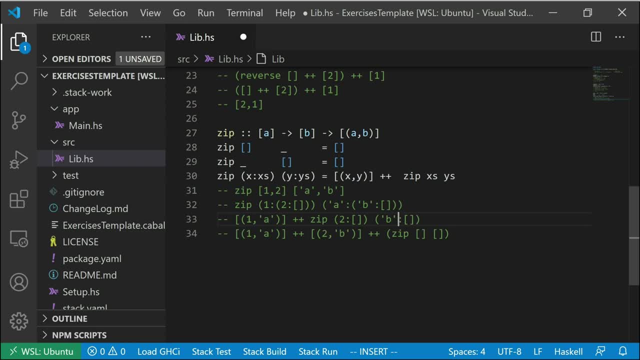 whoops, i think that should have been okay. and then once we got to this case- and it would have been the same if this list or this list was bigger than one or the other- once we get to this case where either of them is empty list, then we're just adding the empty list back right and we end up with a. 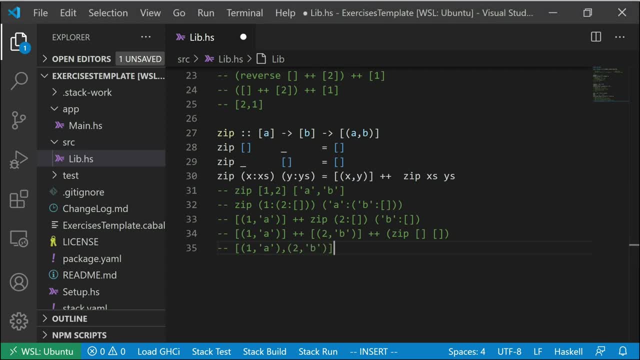 two b. okay, let's try an even trickier example than this. so the drop function takes an int and a list and what it does is it removes the first n elements. okay, whatever this int is, it removes the first n elements from the list. so we have two scenarios here: drop and empty list, drop and axis. 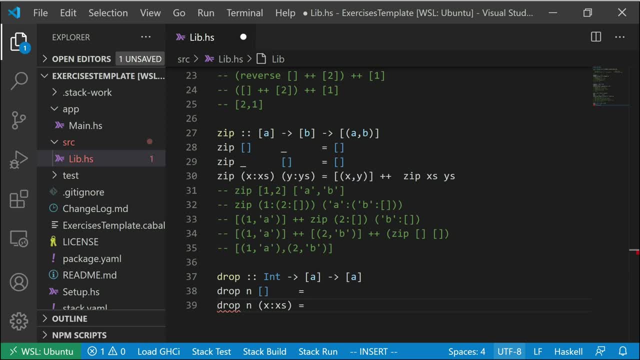 so how are we going to do this? so first of all, we should check how many things we have to remove from the list. so if we have, if we're at zero, like, let's say, if we only need to remove zero things from the list, well, we actually don't. 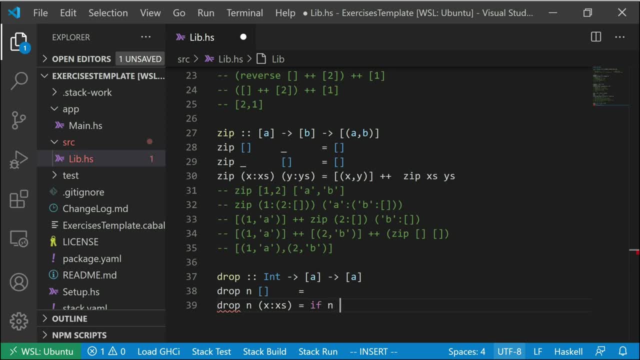 have to do anything to the list, right? so if n is greater than zero, what we'll do then we'll have the recursive case. so that's going to be drop n minus 1 from x's. so what we're going to do is we're going to, we're going to move through this list. 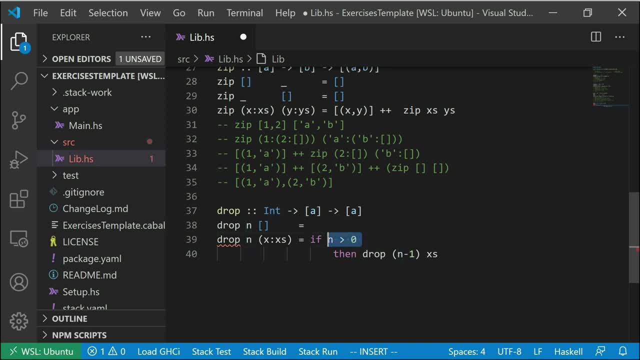 and as long as n is bigger than zero, then we're just going to drop n minus 1 from the rest of the list. but if n is 0 or negative, which will just assume to mean also the same thing as 0, then we'll just 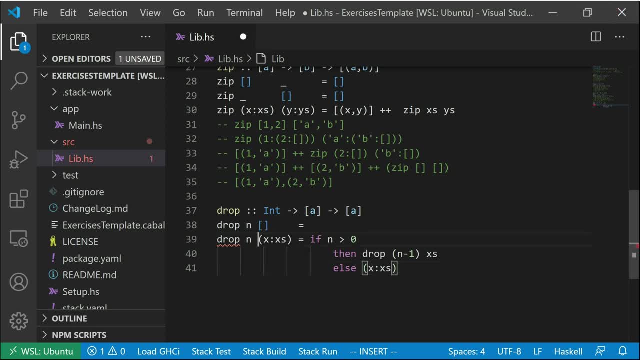 return the list as is. so like what would drop 0 from x-axis be? it would just be the same list x-axis. however, if we get to the empty list, what are we going to do? like if somebody says, drop five things from the empty list, what would you do? 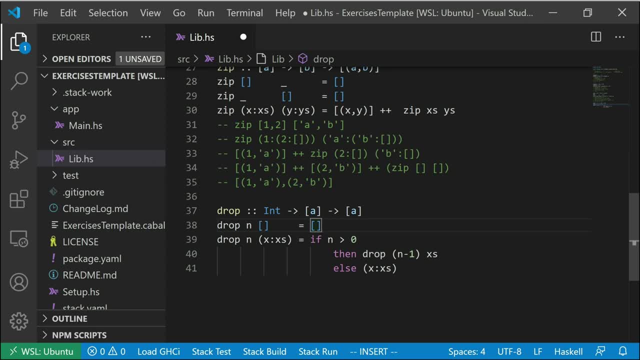 you would just return the empty list because you can't drop any more things from it. okay, so if we were to run through a little example, so we drop one from one, two, so this is going to become. it's just going to check: is this bigger than zero? yes, it is so. 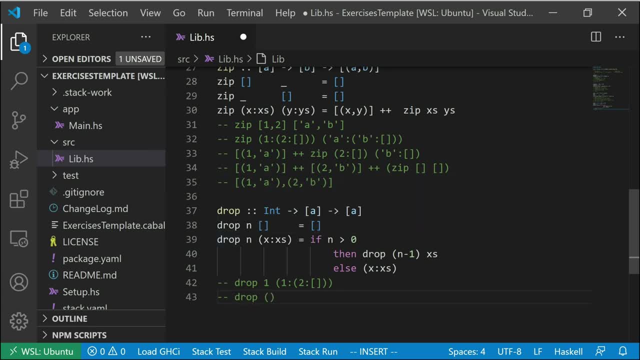 it'll just become drop one minus one, which is of course zero, and it's going to call this on just axis here, so it's going to be two empty lists. and then, when it gets called again, now that this is zero, okay, it's going to return x-axis, so it's just going to return the list of two. 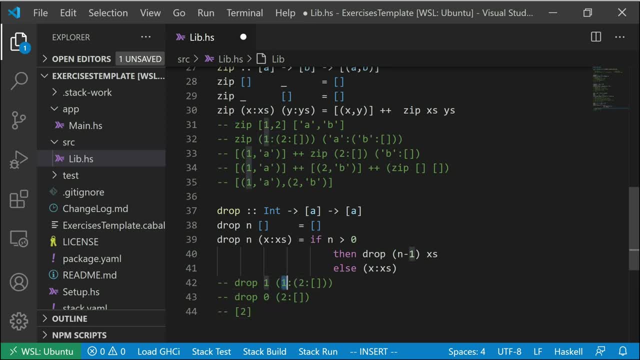 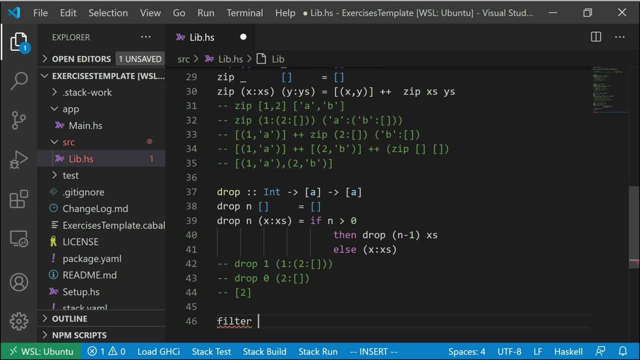 which is exactly what we want here. okay, we want to take one off of the list of one two. nope, we actually could have used guards instead of the if expression here, but the if expression worked well. but another example: a function that is going to have to do something on a conditional and then recurse is the filter function. so the filter. 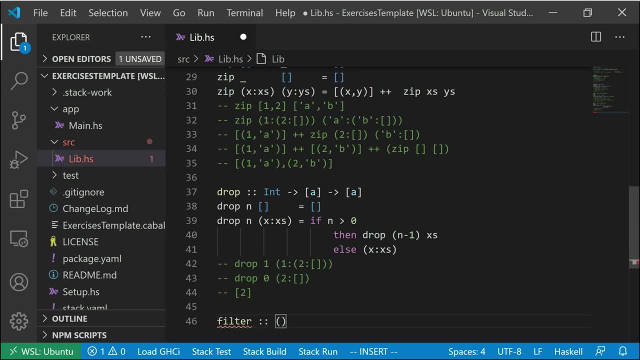 function. it's actually going to take another function as its first argument and that function is going to take an a and return a bool, and then it's going to take a list of a function and then it's going to return a list of it. so basically, it's going to filter a list. 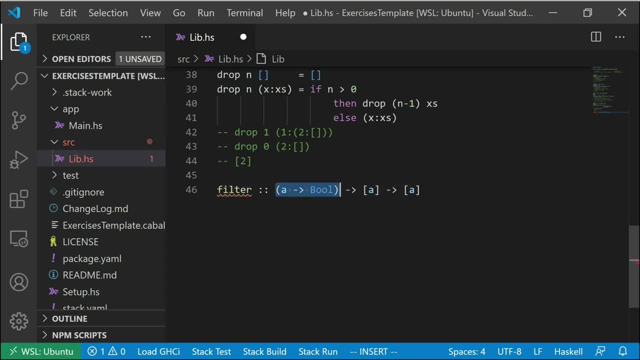 based on whether or not it's able to satisfy this function. so if the element inside this list returns true for this function, it'll keep it in the list, but if it returns false, it'll get rid of it. so we call the function, let's call it p and the list: we're going. 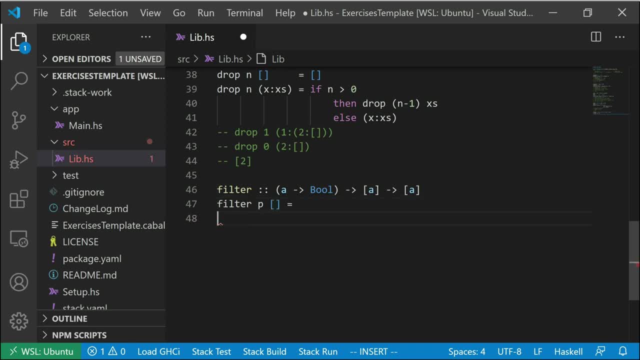 to pattern match over and we can start at. let's start at the base case here. just because it's so straightforward to go about how we're going to filter an empty list again, it's just like: drop, we're not, we're just going to return the list. now the recursive case, what we're going to do. 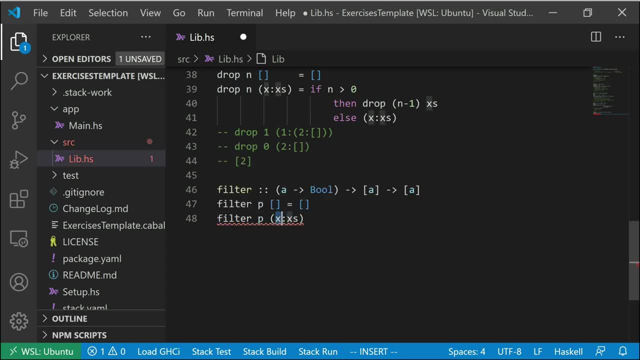 is going to depend entirely on what the result of p of x is. so let's use a guard here and just put p of x and that's all we need to put, because this is going to return true or false, and we're and we're testing for true or false, and so either p of x is going to happen or otherwise. 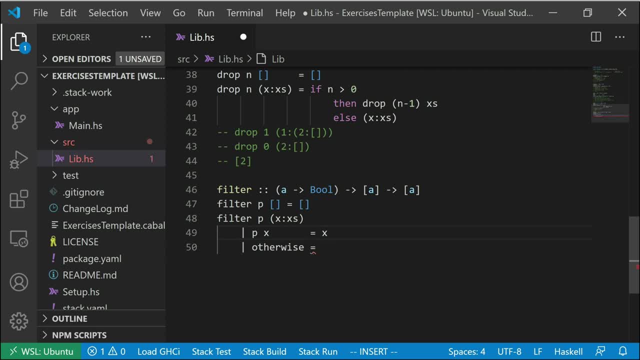 so if this is true, what we're going to do is we're going to rebuild the list, so we're going to say x colon, and then we're going to filter the rest of the list, filter p of x's. but if this isn't true, well then. 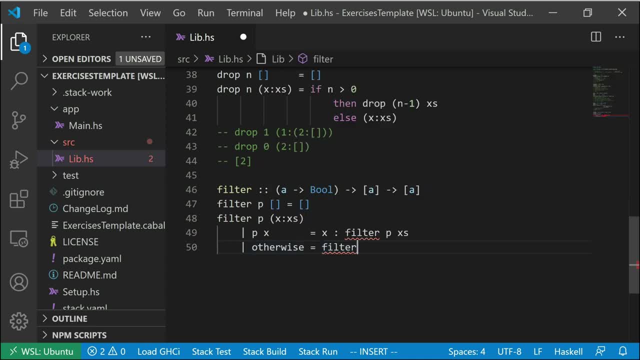 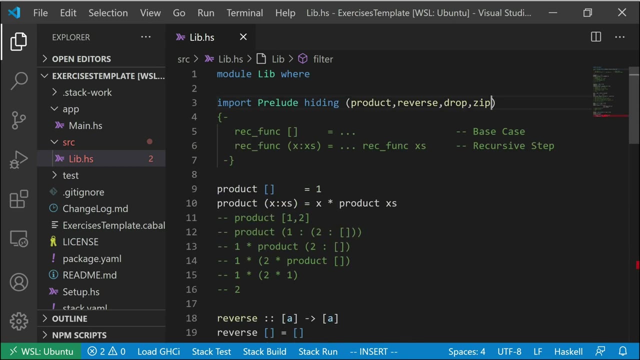 what are we going to do here? we're still going to have to pull filter, but this time we don't need to include this x here, so we're just going to do the same thing: filter p of x's, but not add x to the list here. okay, and just all of these functions. 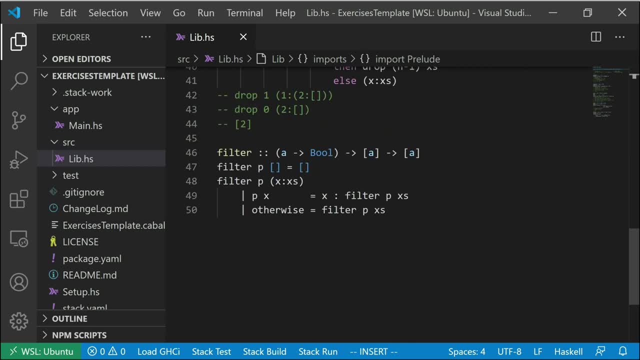 we almost might as well just get rid of the whole prelude at the rate we're going. okay, so so filter. if we went through an example of this, what would be a good example? filter. and we would filter a list to see if they are, even say we have a function. 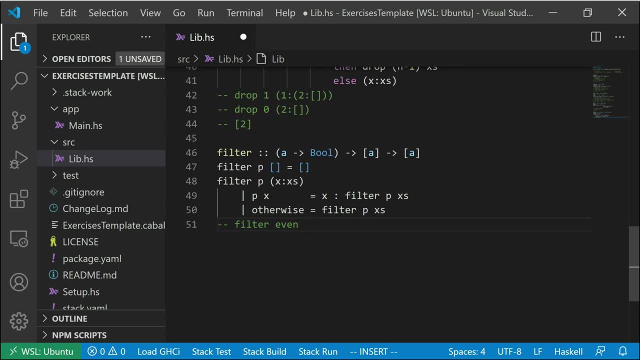 that works with evens. it tells you if a int is even or not. so we're going to say filter even the list of one, two, three, and then say filter p of x, and then say filter p of x and then say filter p of x until that position can be solved. 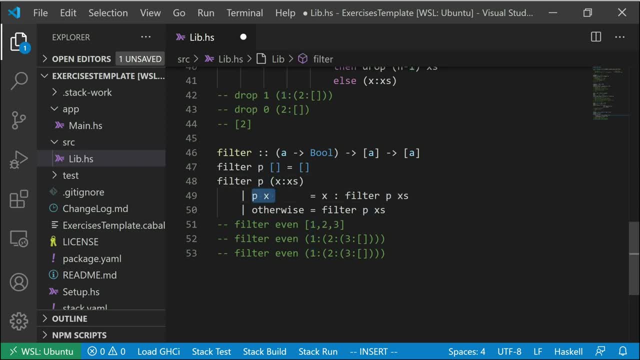 okay. so this is going to become. it's going to start with one, and what's it going to do? it's going to fail. p of x. so p of x is going to be even okay, one and one isn't even so, it's going to just call. 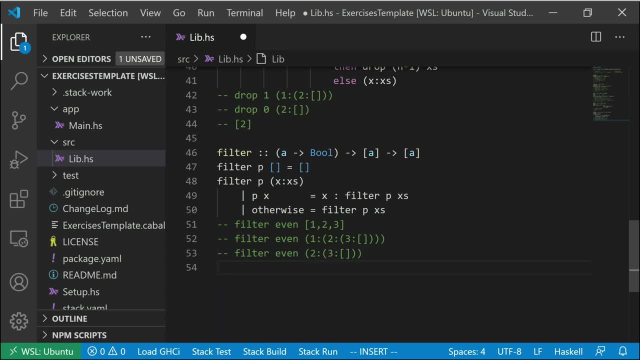 going to be on. And then what's going to happen? Well, now it's going to call even on 2, and this time it is going to keep it. It's going to say: 2 colon filter, even 3 colon empty list. 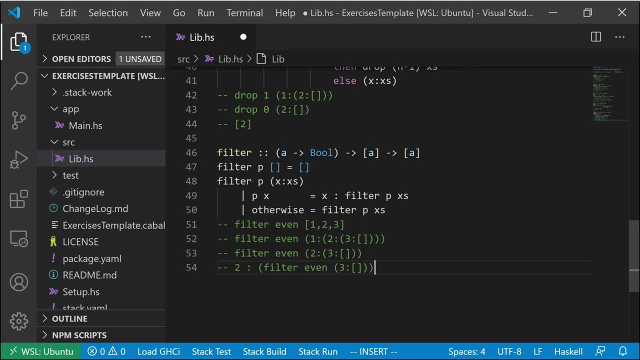 Now this gets called, and guess what? Even of 3 doesn't keep. it Goes to this scenario. So we'll just run it And then we're at the empty list. and what are we going to return? Just the empty list. It's going to be 2 empty lists, which is the same thing as just a list. 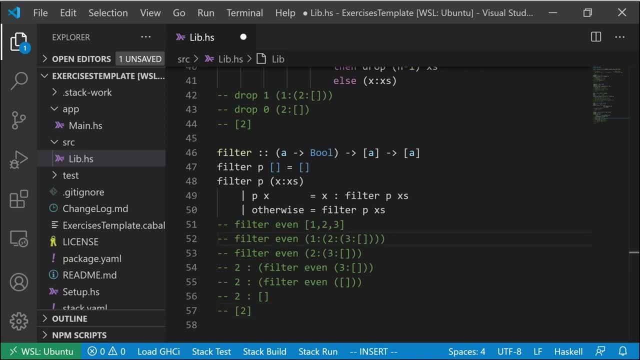 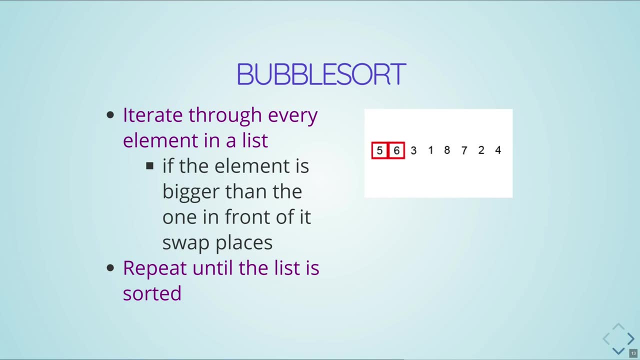 of 2.. Okay, and that's filter. Okay, let's take a look at what's possibly the most popular intro algorithm ever: the bubble sort. So the bubble sort is a sorting algorithm. What it does is it takes like a list and it makes sure it goes through the list and then it 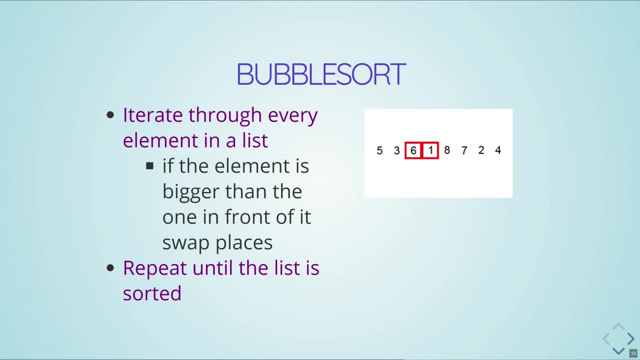 makes sure all the elements in the list are sorted, that they all come in order. So the way it does this is it's going to iterate through the list and, just like inside this GIF here, it's going to check adjacent elements. So it's going to check that for every element. 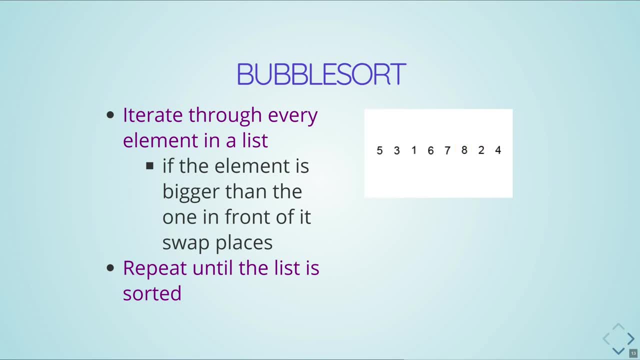 is the element in front of it smaller than it? Okay. if the element in front of it is smaller than it, then they'll swap Okay, and it'll move through the list doing this, and you'll notice by the time it. 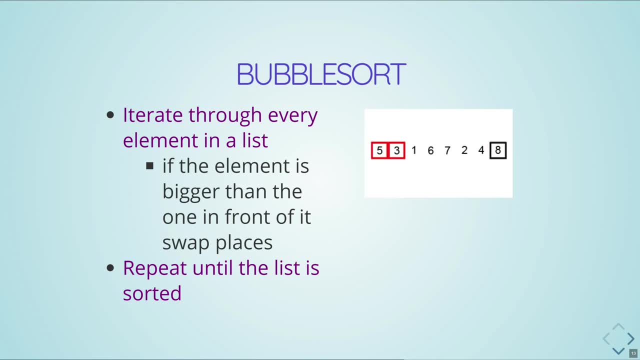 If you start at the first element like this and you just keep moving through each element, moving all the way through the list, by the time you get to the end of the list, it's still not sorted. However, if you repeat this over and over and over again, eventually it 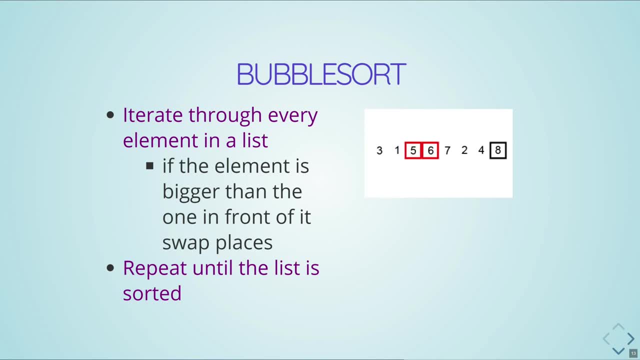 will be sorted And in fact it will only take at most the length of the list repetitions of this. So you'll have to move through the entire list and then move through it again, move through it again. the length of the list times at the most to arrive at the end of the list. 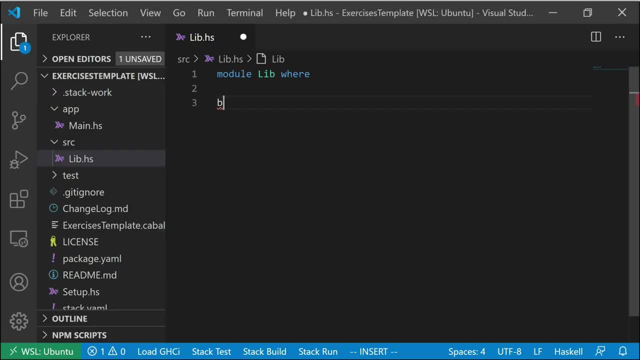 Okay, let's start off with creating a function bubble, And what bubble is going to do is it's going to move through a list. let's say x. x is here and it's going to compare x to the thing in front of it in the list. Now the problem here is: okay, we have the first thing in the list. 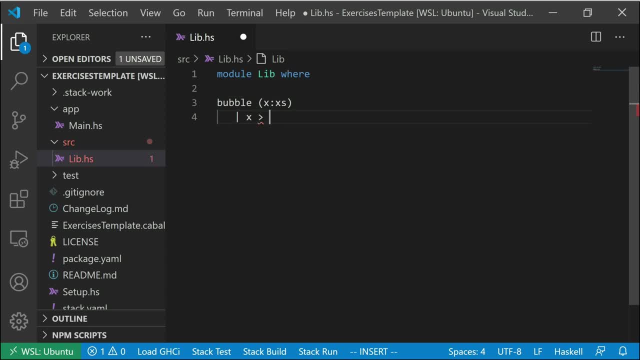 and we have the rest of the list. But we also need the second thing in the list. We want to say if x is bigger than the thing that's in front of it, right? So let's switch up this pattern match a little bit And let's make this x zero, x one x's. So 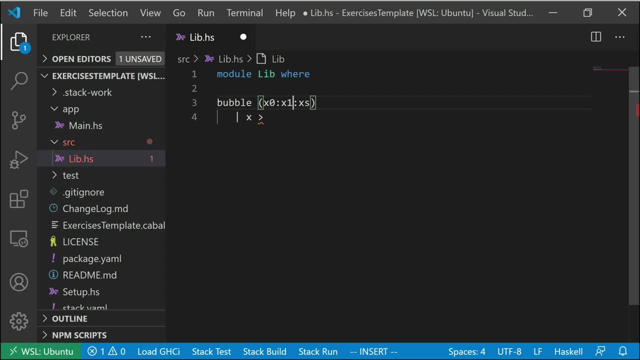 this is the first thing in the list, the second thing in the list and then x's. So you'll notice this pattern match is only going to work if there's at least two things here. but we'll get back to that. So we'll say: if x zero is bigger than x one, then what are we going to do? we're. 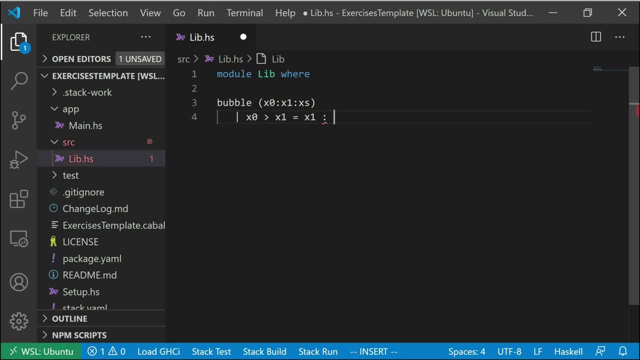 going to put x one in front and then rebuild the list, continuing with x zero, x one and then x two. So now we're going to call bubble, we're going to rebuild the list with x zero now moved in front of x one here. So we moved x one to the back here And otherwise we're just going to leave. 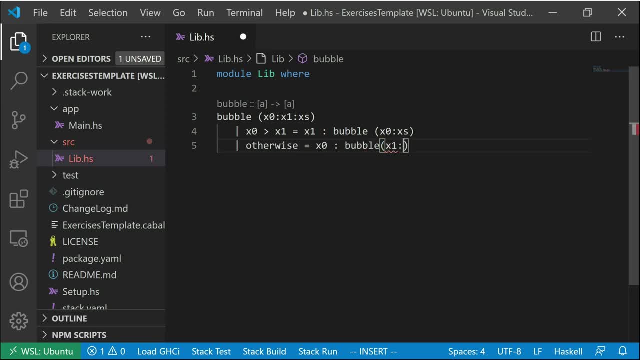 things as they are, we'll leave x zero there And we'll continue moving through the rest of the list. So if x zero is not bigger than the thing in front of it, then we're going to rebuild the list and we just call bubble on the rest of the list and we leave x zero alone where it is. 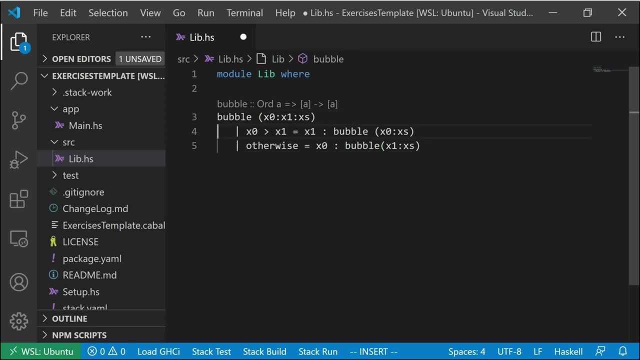 So we're going to do this As long as there's two elements of the list. this is what we power match to as long as there's two elements of the list. So now we need to take care of the scenario. What if there's more? What if there's one? So we get- we can try out- two scenarios here. What if there's one? 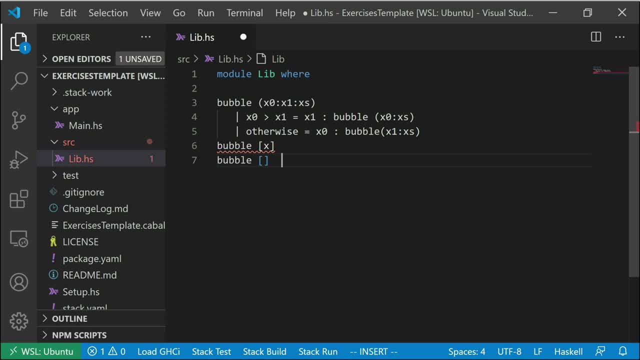 thing in the list? And what if there's nothing in the list? So if there's nothing in the list, this is, this is an easy one. We'll just return the empty list. How do we, how do we sort the empty list? the empty list, sorted is just the empty list If there's one. 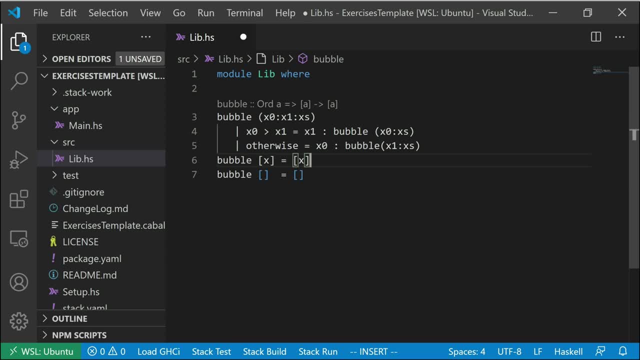 thing in the list. oh, guess what? we're also just going to leave it alone. Okay, how do we sort a list of with one thing inside it? we just leave it alone. it's just a list of one thing, And so. 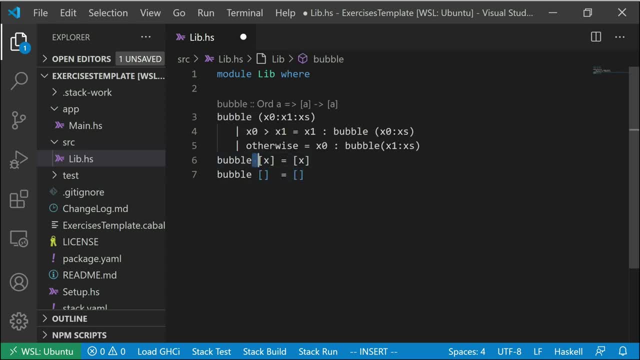 actually we can shorten this up here. instead of power matching to these two cases specifically, we could just make sure it's underneath this pattern And then be like anything else. any other pattern X is here. we'll just leave it as it is. Okay now. 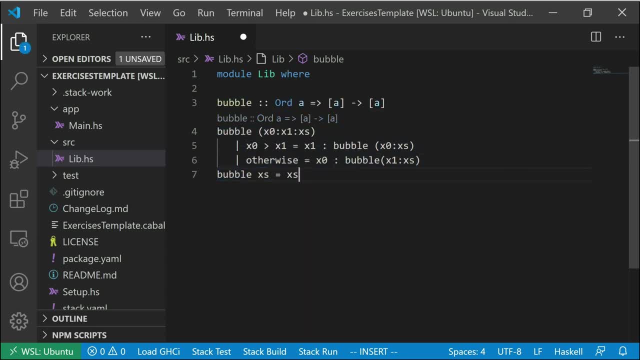 this is. this is part of bubble sort And you'll notice it'll work on any list of a, as long as it's part of the order book class, which basically is just saying, as long as you're able to do this comparison, they one thing is greater than the other. 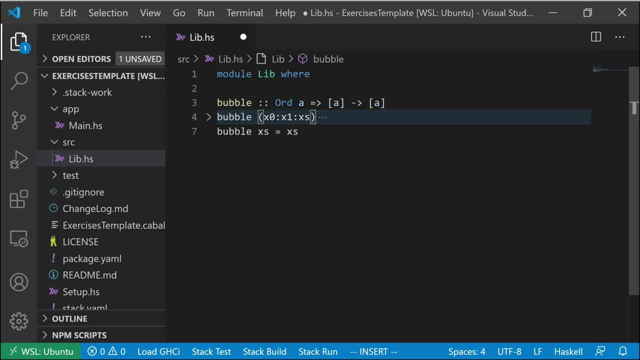 Okay, but you'll notice this isn't enough. This function alone isn't enough to actually sort something. To actually sort this, what we need to do is we need to call this function until the list is sorted. So we could write a function: bubble sort. It's going to take an Xs. Okay, it's going to take some list xs. okay, going to take some list xs. okay, it's going to take some list xs. okay. 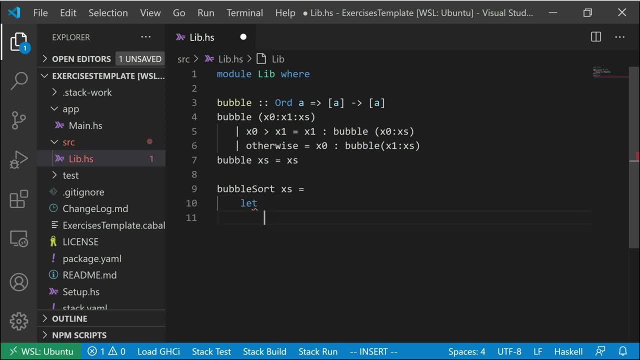 and what it's going to do is say: let x's prime equal bubble x's. We'll create another variable, x's, that calls this function on it. So we'll call the function and we'll get. we'll get some results and we'll say if x's prime is. 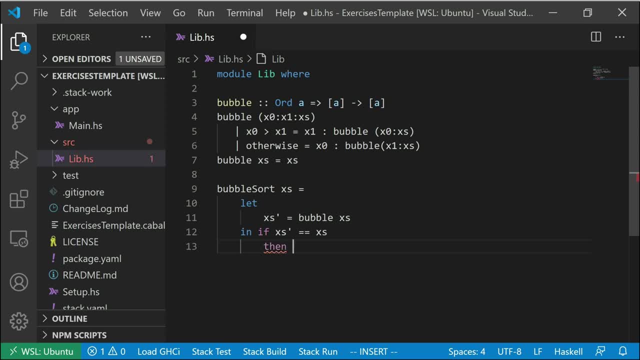 equal to X's then. So, in this scenario, calling bubble on the list isn't going to do anything more. It's already it's. it's just staying the exact same thing. That means we must be done, it must be sorted. So in this case, we will just. 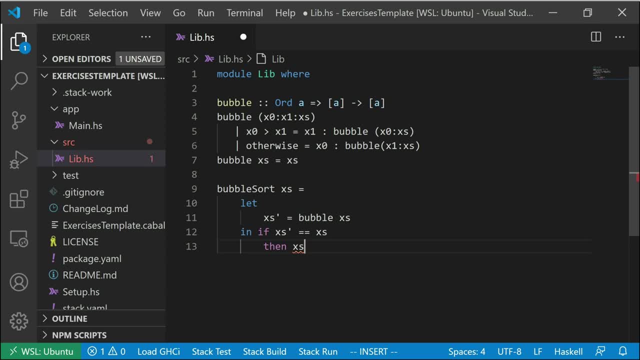 return x's or fp's prime, it doesn't matter, do the same thing. we'll just return it and be like, okay, this is our sorted lips, but if it's not the same thing, then we don't know if we're done yet. So if we don't know if we're, 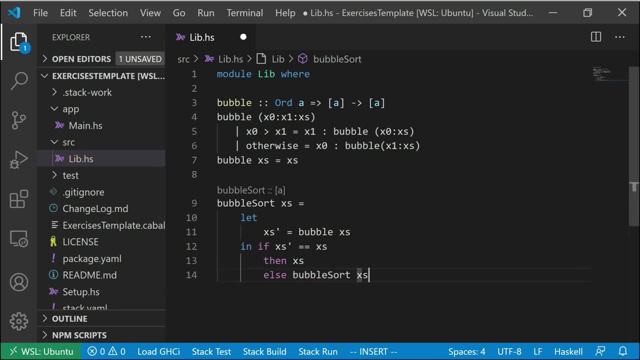 done yet, then what we'll do is we'll just call bubble sort again on x's prime. now, okay, make sure to call on x's prime, because we need to call on the thing we're updating. that's been updated, and now this function altogether is sufficient enough to actually sort your list, and it'll do. 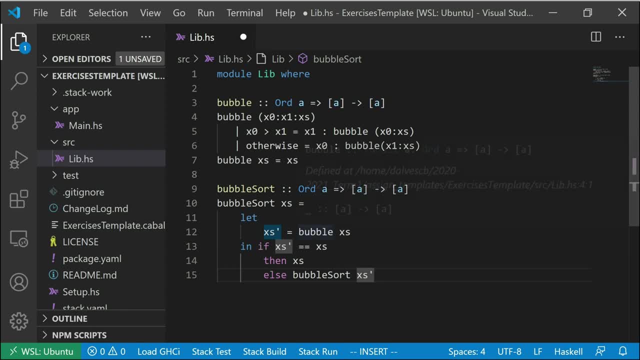 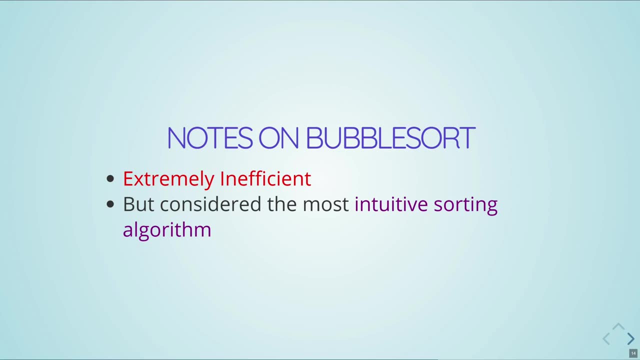 it in at most the length of list calls of bubble. however, it might do it in less. just a note on bubble sort, now that i've taught you it: uh, never use it please. it's extremely inefficient. basically, the only reason people even acknowledge its existence is it's considered the most intuitive. 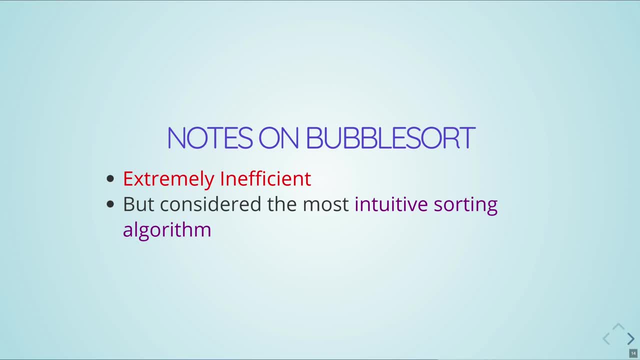 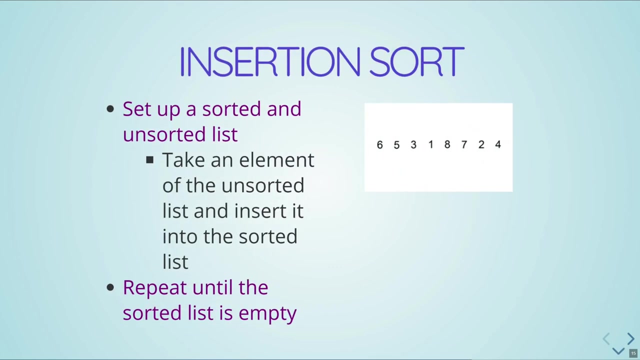 sorting algorithm. so if you were to get a group of elementary school students together and somehow trick them to developing a sorting algorithm, what would be the most likely sorting algorithm they would come up with? probably the bubble sort. however, you never, ever, want to use it. another type of sorting algorithm is the insertion sort. 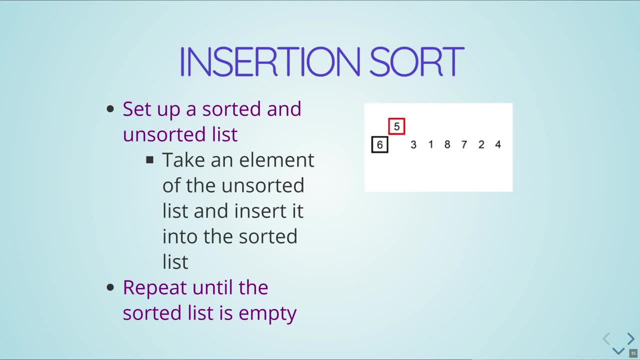 so this is an algorithm. it's going to do the same thing as the bubble sort: it's going to sort the list, but it's going to do it in a different way. so the way the insertion sort is going to work is it's going to set up a sorted and an unsorted list, and the trick is that at the beginning, the 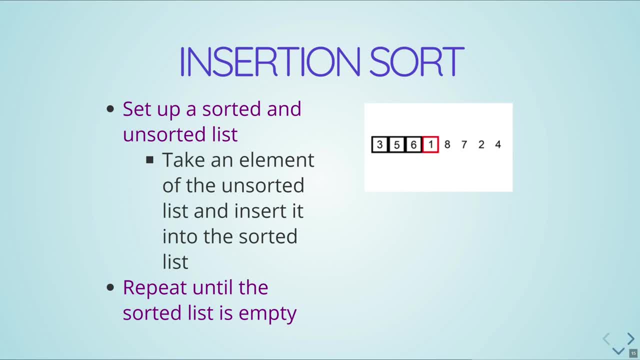 sorted list can just be an empty list, and then what you do is you sort it in a different way. you take an element, like in this gif here is showing. you take an element and you insert it into the sorted list, and the idea here is: because you know the list is already sorted, you just kind. 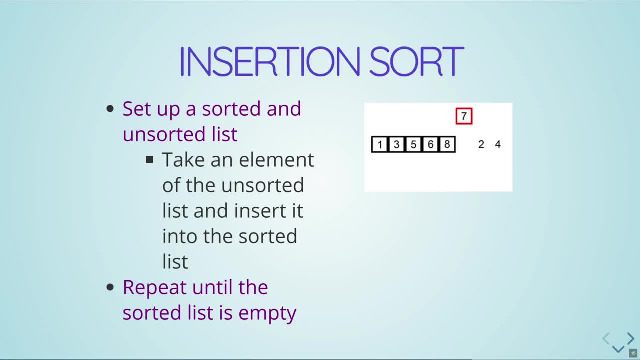 of move through the list and as soon as you find the spot where it's like oh, i'm bigger than this guy, then you insert it in. okay, so you just do this. you move to the list and insert every element of the unsorted list into the sorted list and eventually you just wind up with one big sorted. 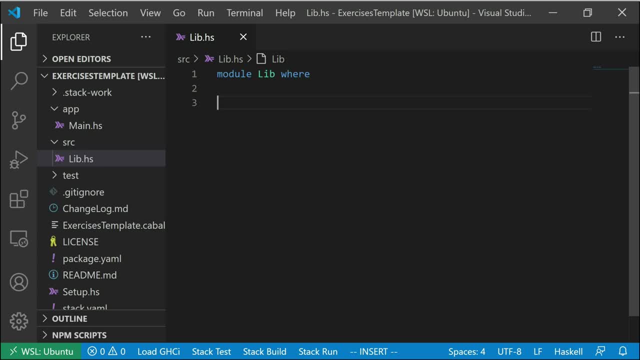 list. okay, let's try making the insertion sorted in haskell. so, to start off, we're going to create a function insert, and it's what it's going to do is it's going to take a variable x and it's going to insert it into a list, wise. and the idea here is we're going to assume wise is sorted and insert x. 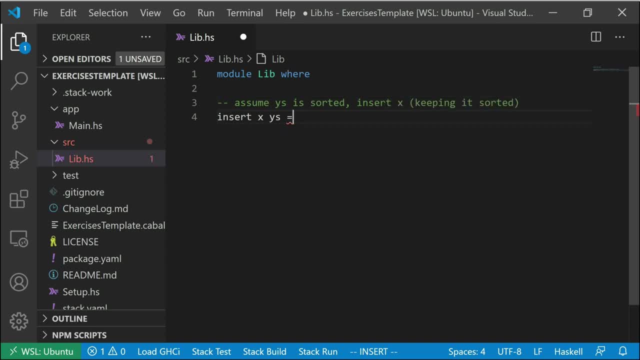 keeping it sorted. so to do this, let's use a guard. what we're going to do is we're going to pattern match on wise and using guards. it's going to be similar to the bubble sort. we're going to compare x to the current element of the list and if it's smaller than it, okay, then that means. 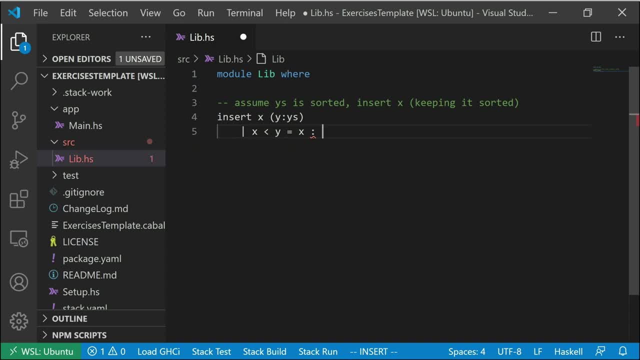 we can put it in front of wise, and it'll still be sorted, because y wise is already sorted. on the other hand, though, if x is bigger, then what we're going to want to do is we're going to want to take y here, and then we're going to not not quite do this. what we need to do is, um sorry, this. 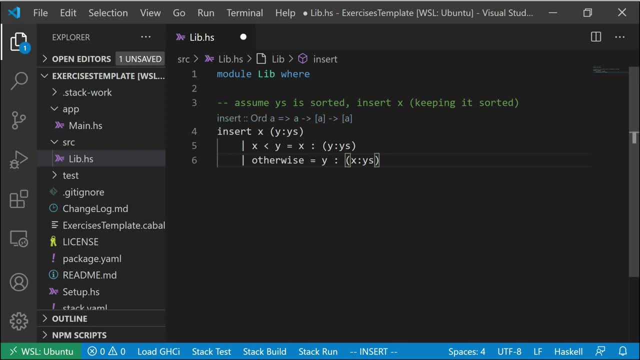 needs to be wise. what we need to do is we need to continue inserting x into the rest of y's here now. so we'll need to insert x into y's. so this way we'll continue moving through y's until we find the y that it's smaller. 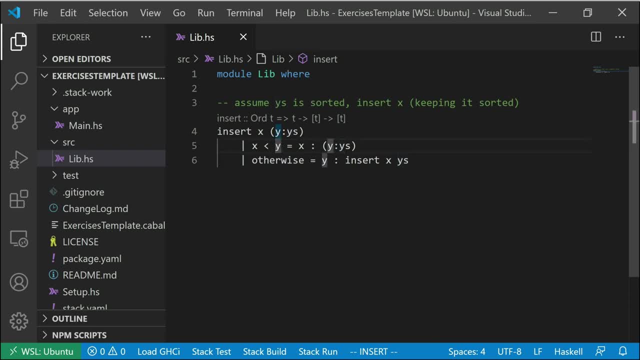 than okay, um, and then insert it there, and if it doesn't find the y that's smaller than then, we'll end up at this case. so we'll end up at the uh, at the other case of insert x, empty list. and what are we going to do here? well, we're just going to insert x. 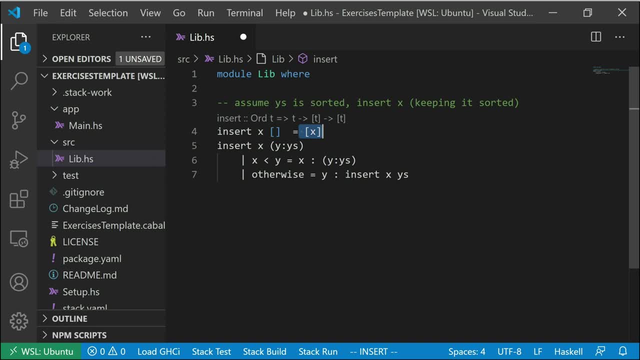 into the empty list here. we're just going to make the single thin list of acts okay. and now that we got this list, what we need to do is we need to write a function now, insertion sort. and the way insert sort is going to work, it is going to iterate through a list: x, axis. 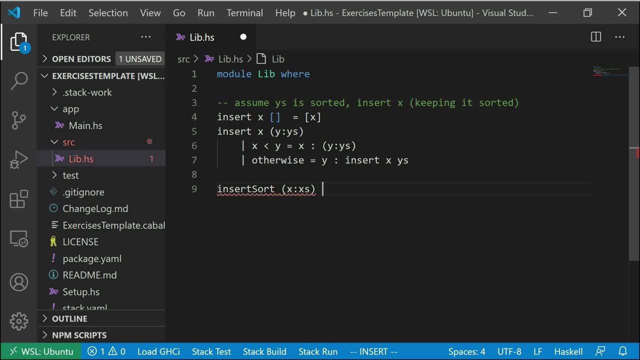 okay, and what it's going to do is it's going to insert x into the sorted list. x's here. so what's what's happening here? so what we're doing is, um, we're taking the list the, the head of the list- x here, okay- and we're inserting it into an already sorted list. we know it's an already sorted. 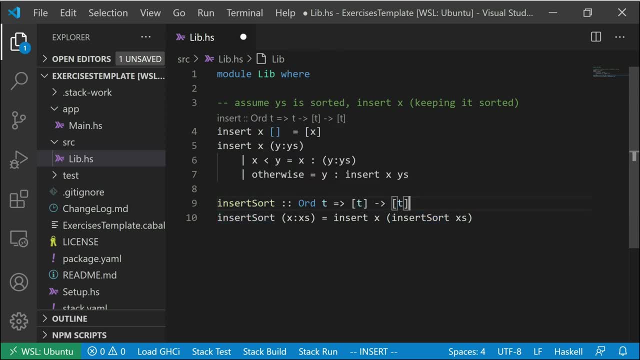 list because we're calling insert, sort on it, right, and we're going to keep doing this until we get to the empty list here. and then, once we get to the empty list, we can just return the empty list because, guess what, the empty list is already sorted. 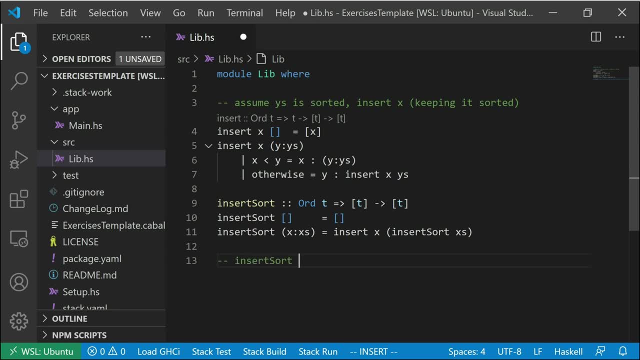 so what we're going to do here is, let's say, we have insert, sort the list of four to five. okay, Liz is going to evaluate, you going to evaluate into insert for them to start going to five. you know, I'm actually gonna skip a step here. you can imagine eventually it just turns into insert. you insert five. 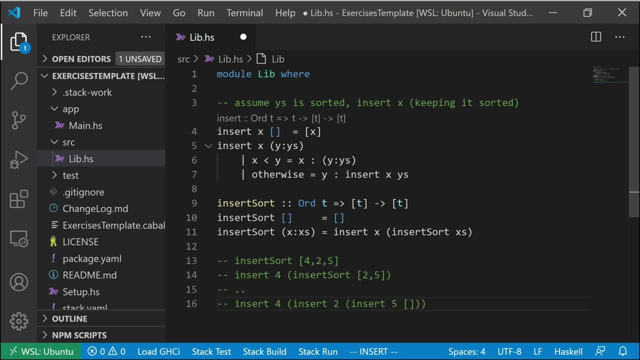 into empty list. okay, so after all of this, these recursion, all of the insert sort recursions have happened. you wind up with something like this, and then we go all the way back up inserting one of these things at a time into the empty lists until you wind up. 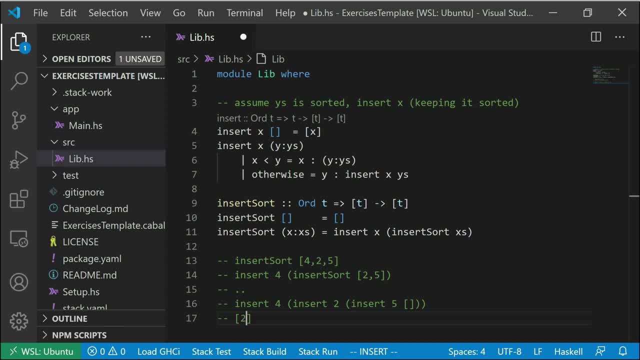 with the sorted lists. so two, four, five. okay, because you it inserts, go through this one second time. so insert five empty lists here turns into just a list of five, which then turns into two, five, which then turns into two, four, five to four, five. okay. let's talk about one more sort, the Quick Sort. 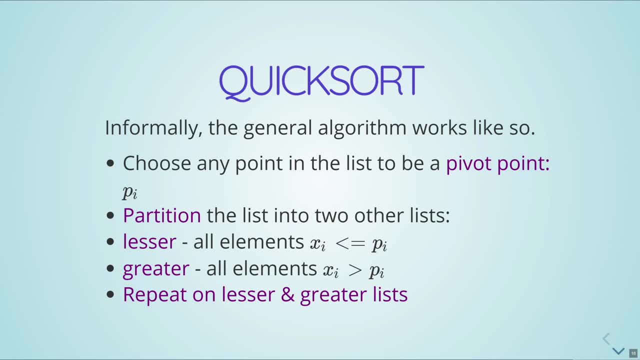 so the Quick Sort is a bit harder to visualize, but it's not that un-intuitive. so the way it works basically is that you choose a pivot point in the list. so this pivot point could just be any element in the list. they could just be the first element you pull out of this. it doesn't. 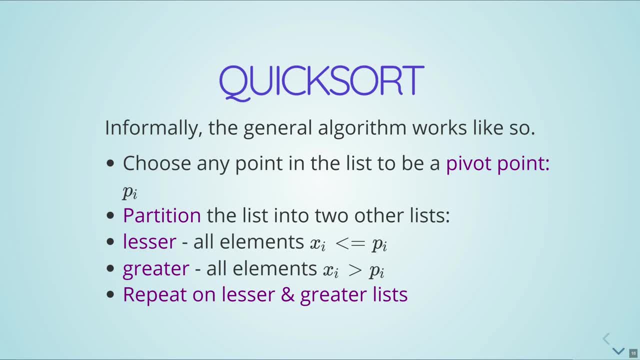 matter. and what you do then is you partition two other lists, so you create two other lists from the remaining list of all the elements that are smaller than the pivot point and all of the elements that are greater than the pivot point, And then you repeat this operation. 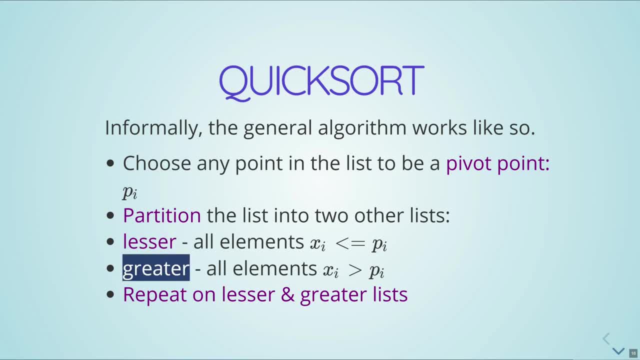 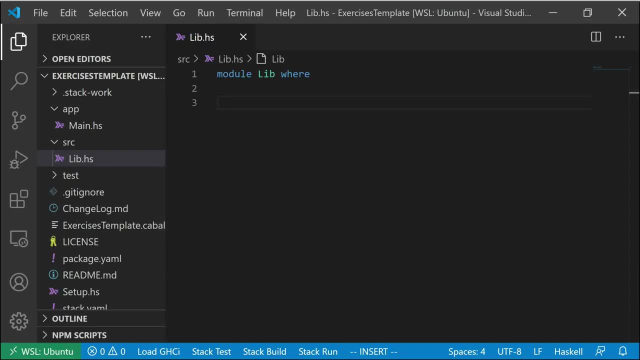 on both the lesser and greater list that you end up with and eventually just kind of put it all together into one big sorted list. So how are we going to implement this in Haskell? So we'll create a function, qsort, and we'll just start off with the base case of the empty list equals empty. 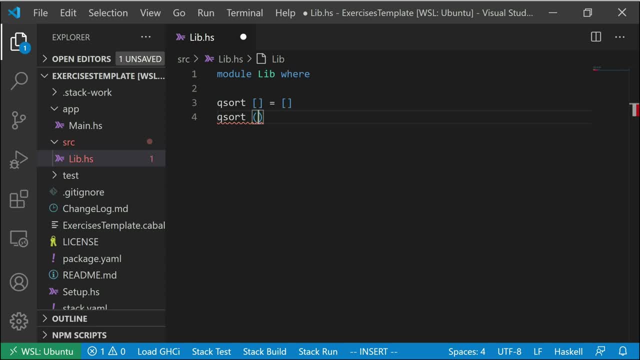 list and we'll pattern match and what we'll do is the pivot point will just be the first point of the list. so we'll pattern match on the list and the pivot point will just be the head of the list, the first thing in the list. And what we're going to do is we're going to have to divide this up. 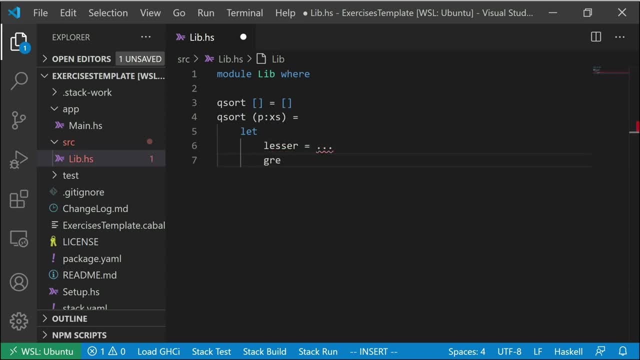 into lesser and greater, Okay, and once we have. so we'll just leave this alone for a sec. we'll define these in a second, Once we have the lesser and greater list. what we're going to do is we're going to perform the quicksort on the lesser list and the greater list and put it all together. 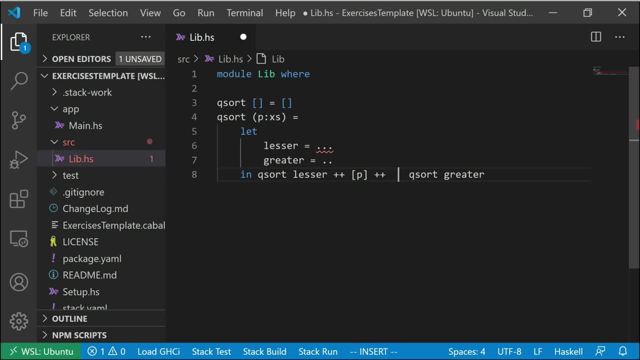 with p in between. Okay so? so this way we'll sort one partition of the list, the other partition of the list and p will be in between. Now there's a few ways we can go about implementing how to partition things into the lesser and greater list. One way that actually isn't that efficient. you probably 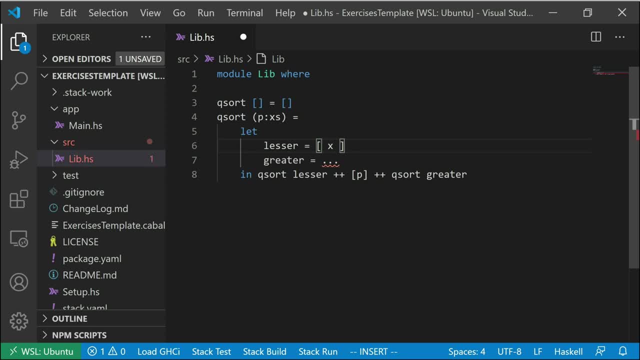 shouldn't do it, but just kind of looks really nice, and so it's a good place to start out when learning about this algorithm is to use list comprehension. So we say: x comes from the list x's and x is smaller than p. x, x from comes from the list x's and x is greater or equal to p. 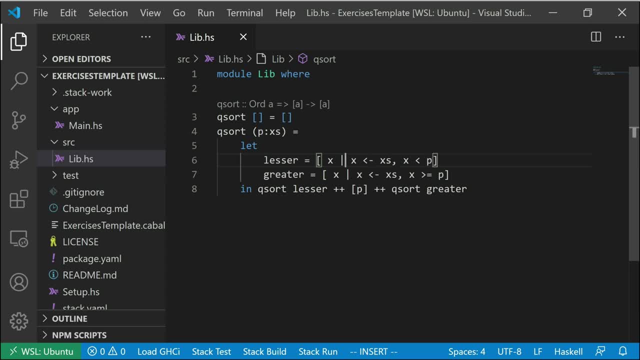 We also could have used, let's say, the filter function. we just said filter x. x is less than p, x's Okay, and there's another option. and then we would have been. we would have done basically the same thing, but with greater or equal to. this should actually be less than or equal to. 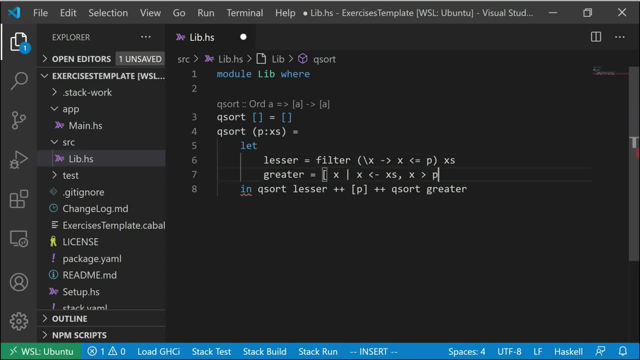 and this should be graded, then it's not. that's actually not a big deal, that really doesn't matter, but this is it. this is all that's required to create the quicksort. So you'll notice it actually has a pretty easy definition inside Haskell. So it's a little bit difficult to examine the evaluation of quicksort, but the way I like.